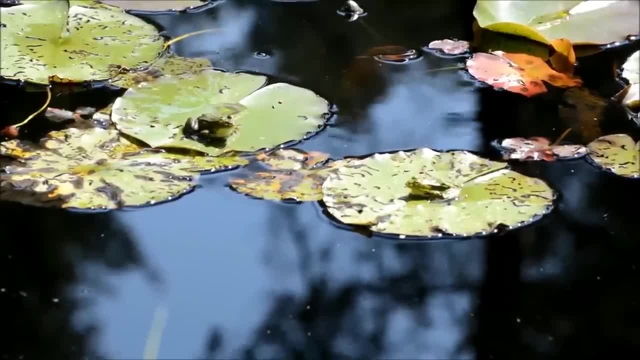 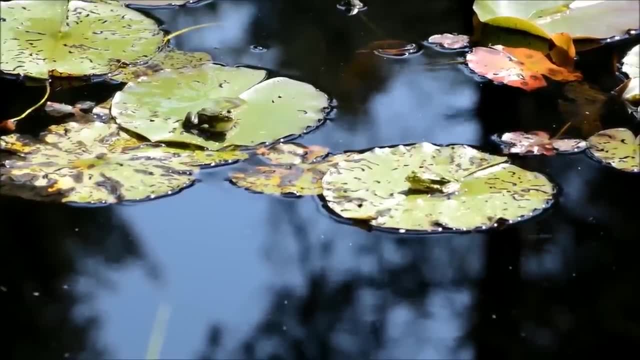 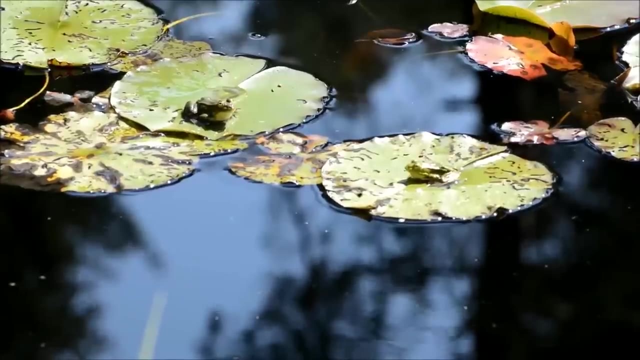 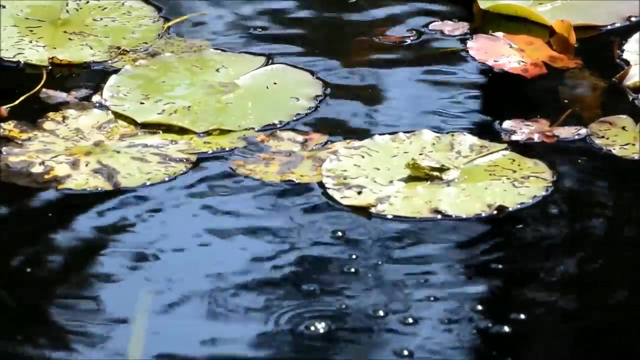 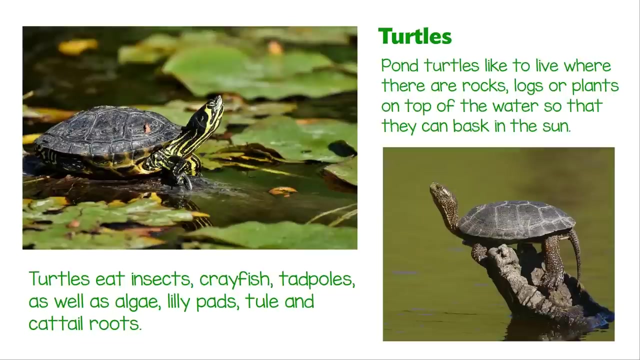 a lot of fruit, like eggs and chicken. The best way to eat is with wine. The best way to eat food is with wine. A little birdy is best in the pond- A little bird-in-the-wild turtles. pond turtles like to live where there are rocks, logs or plants on top of the water. 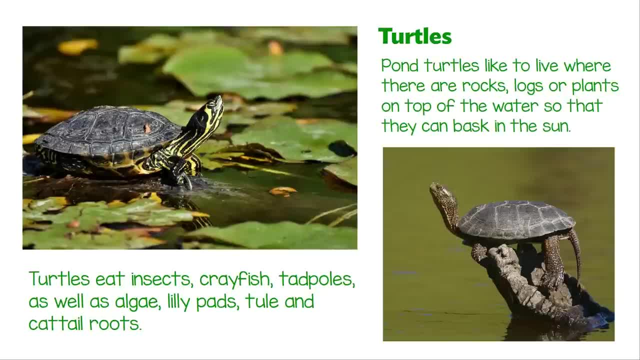 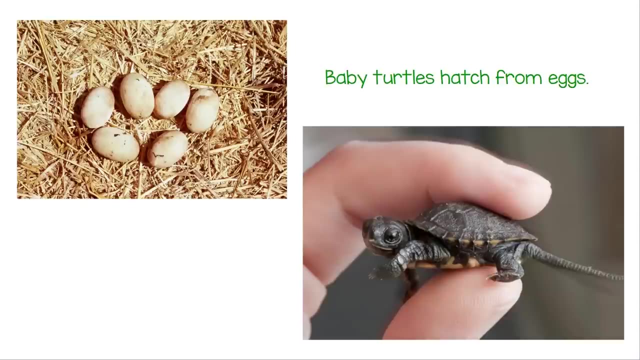 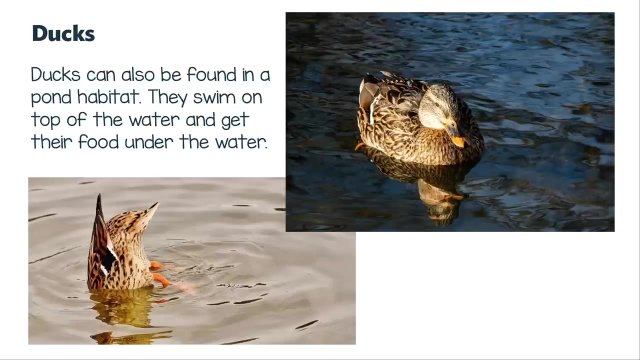 so that they can bask in the Sun. turtles eat insects, crayfish, tadpoles, as well as algae, lily pads, tool and cattail roots. baby turtles hatch from eggs. ducks can also be found in a pond habitat. they swim on top of the water and get their 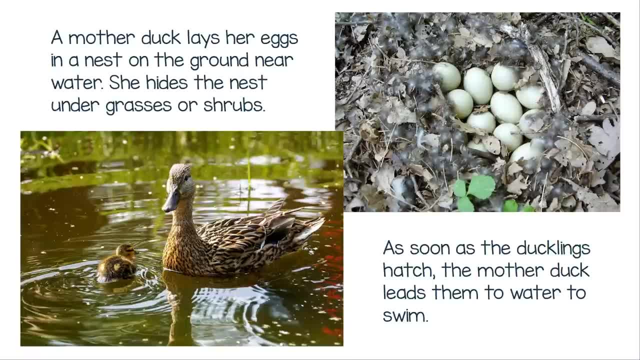 food under the water. a mother duck lays her eggs in a nest on the ground near water. she hides the nest under grasses or shrubs. as soon as the ducklings hatch, the mother duck leads them to water to swim. ducks stay dry in the water by 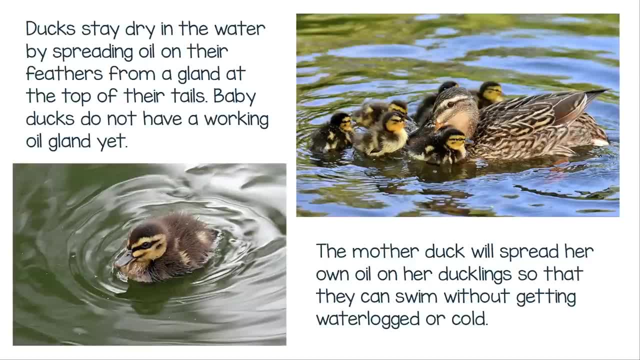 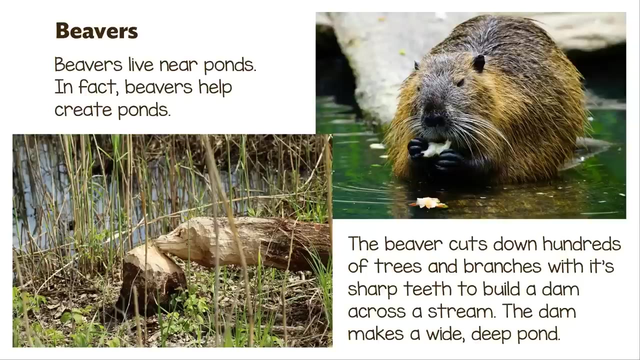 spreading oil on their feathers from a glass land at the top of their tails. baby ducks do not have a working oil gland, yet the mother duck will spread her own oil on her ducklings so that they can swim without getting waterlogged or cold beavers- beavers live near ponds, in fact. 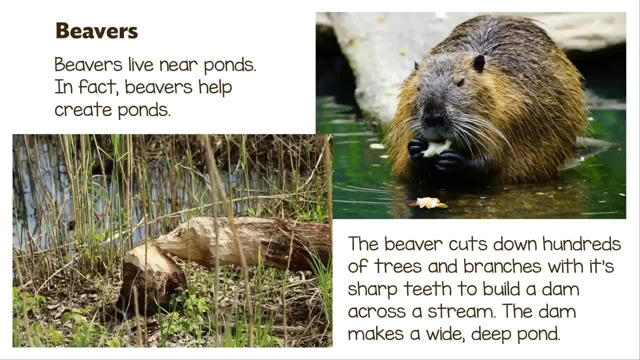 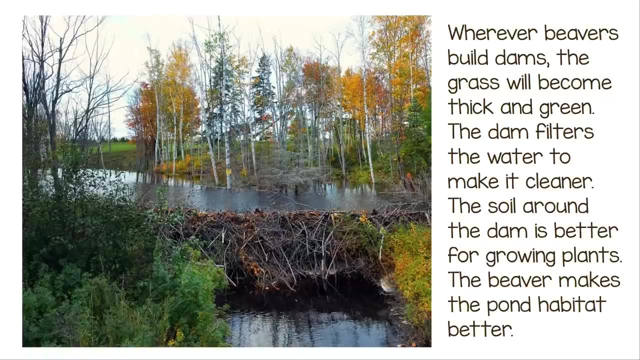 beavers help create ponds. the beaver cuts down hundreds of trees and branches with its sharp teeth to build a dam across a stream. the dam makes a wide, deep pond. wherever beavers build dams, the grass will become thick and green. the dam filters the water to make it cleaner. the soil around the dam is better for.